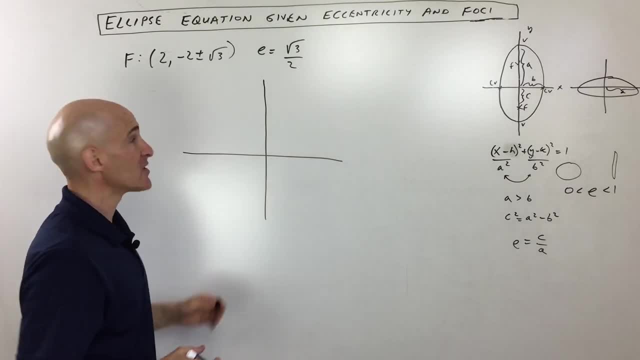 kind of sketch it as i go along and piece the equation together, also as i go along. they're giving us the full side, which are going to be a little bit more complicated. but i'm going to just kind of sketch it as i go along and piece the equation together also as i go along. they're. 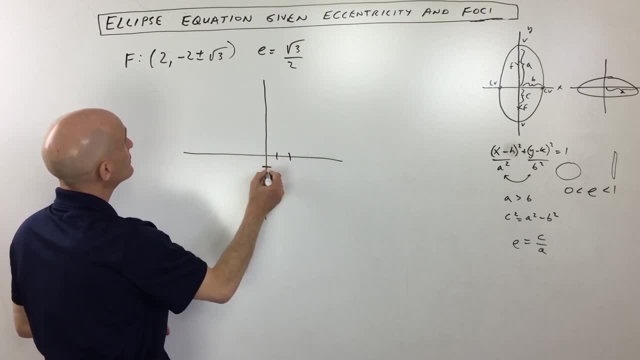 giving us the full side, which are at positive two, and then it's at negative two plus or minus square to three. so what that means is that from here we're going up square to three, which is about 1.7, okay, and down 1.3, which is about 1.7 from from there. so the these are your foci halfway. 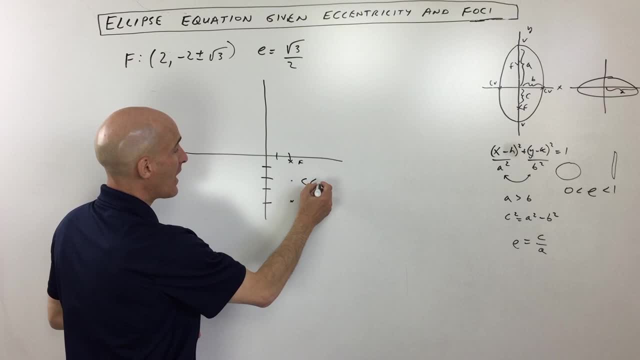 between your foci. that's the center point. so you can see, in this problem the center is at two comma negative two, and this distance from the center to the focus is square to three. that's our c value. okay, so you're with me so far. now the eccentricity is equal to square root three over. 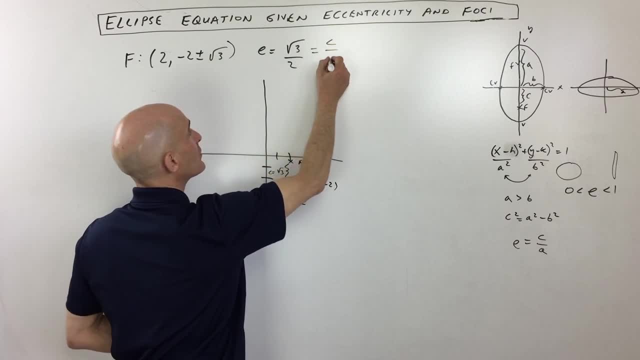 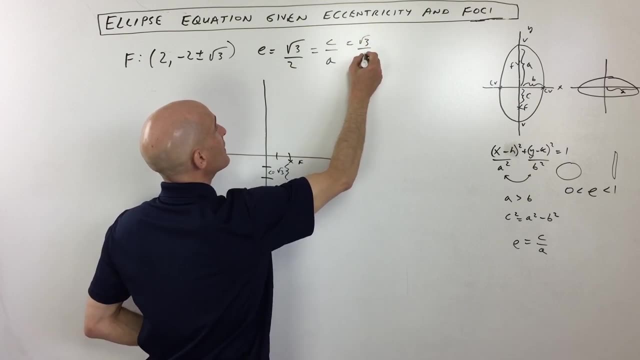 two. but remember, eccentricity is c divided by a. so we have a little equation here. we already figured out that c is square root of three, so that means that a must be equal to two. okay, so this was kind of an easy one. as far as you know, they kind of gave us a c value. we just had to figure out the. 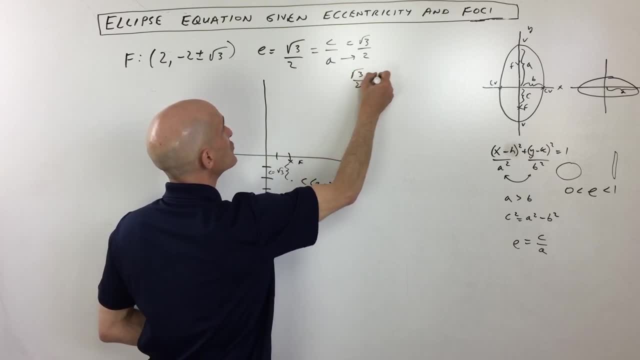 a value. but basically you just have: square root of three over two is equal to c over a square root of three. we're solving for a. you can see that if you cross, multiply, or you can just see that these are equivalent. a is equal to two. now what that means is that from the center to the 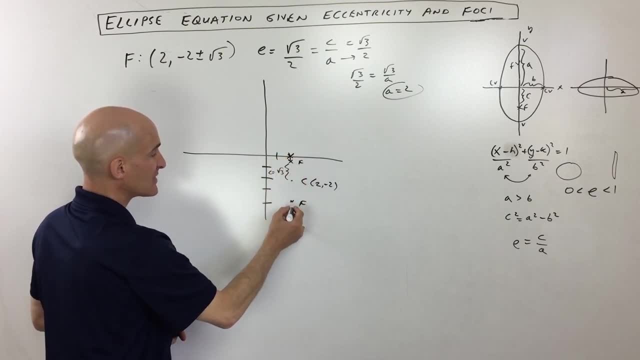 vertex, that distance is two, and then same thing here down two. so these are our vertices, right here, at two zero and two negative four. okay, now, the foci and the vertices are always on the longer axis, the major axis. so you can see, it's gonna be, you know, stretched more in this vertical or this. 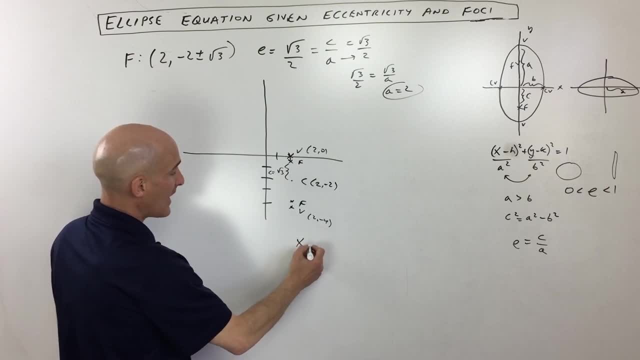 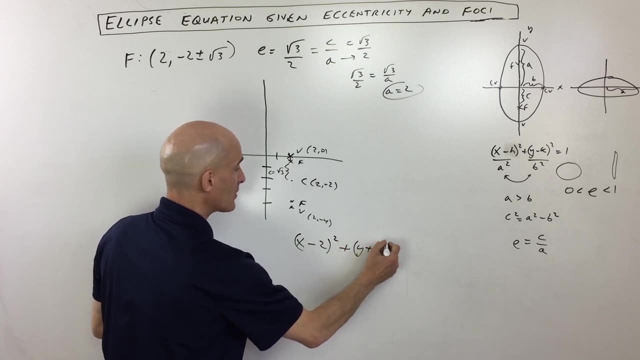 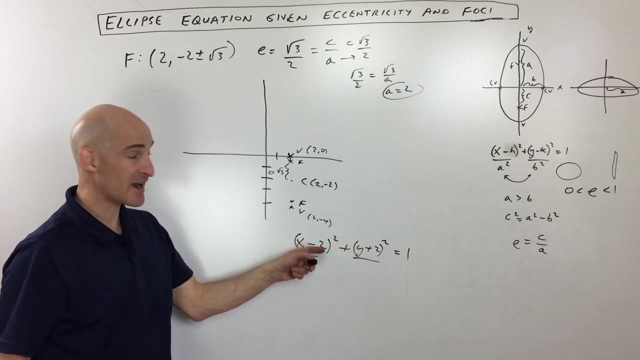 vertical axis. let's see if we can piece together what we have so far. so we've got x minus two squared plus y plus two squared is equal to one. okay, now the reason i put this. this is the center. it's been shifted right to notice. this is the opposite: x minus h. so h is positive two y. 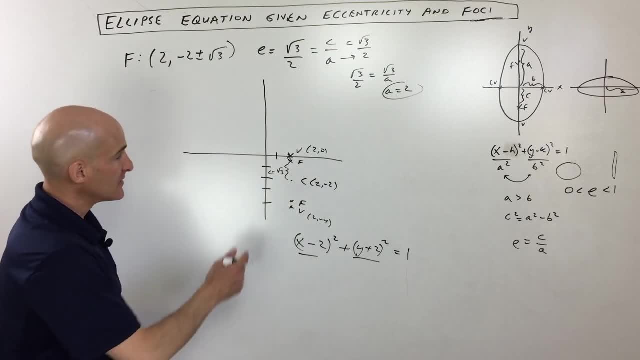 minus a negative two. so k is negative two. we're shifting down two and the distance again from the center to the vertex. that's a. okay now, because i'm going up and down in the vertical liver, or vice versa. you're gonna have a pretty specific spot down in the vertical liver, okay, so you have a. now, because i'm going up and down in the vertical liver and that's what's causing clarity. okay, now then can we- took that- we should be able to do that here at the default. and these dots, parallel shots, cog, function with the ever coin space that really are. what, however, are the sort ofstroke and 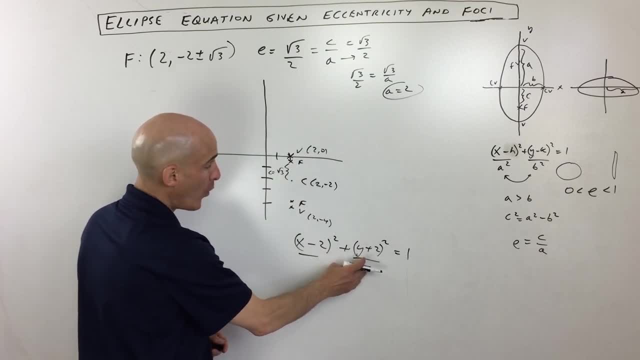 together n the care talks about the entireособ of the hyperverte gustaría direction that a value is going to be underneath the y variable here. that's the y direction, so that's going to be 2, and remember it's 2 squared. so this is actually going to be. 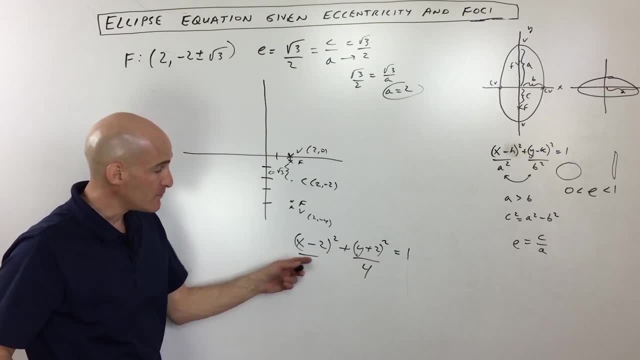 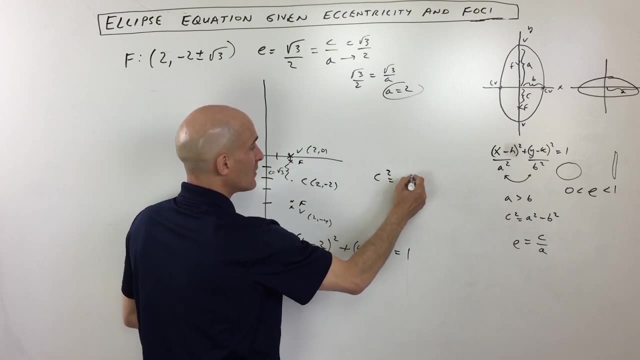 4. okay, now the only thing we're left to solve for is b squared, okay, this denominator, and we're going to use this equation right here. c squared equals a squared minus b squared. so let's see if we can fill in what we know here. we know that a is 2, so that's going to be 2 squared is 4. we know. 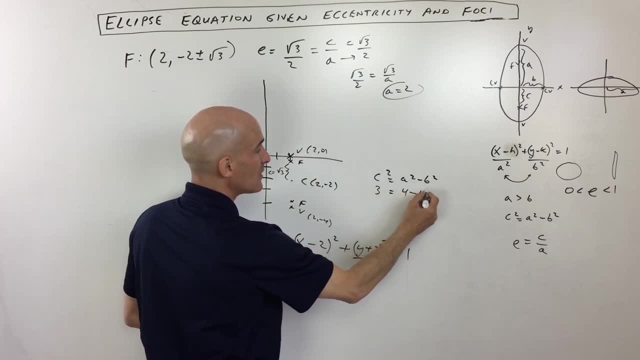 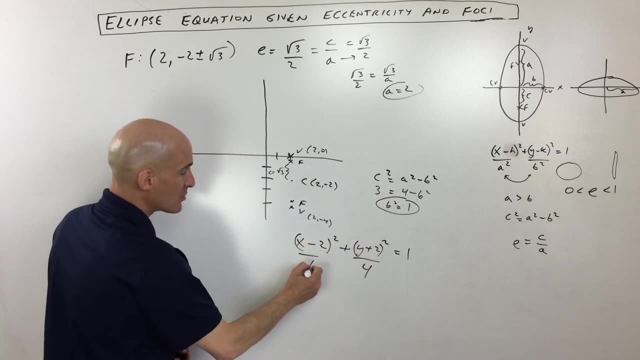 c is square root of 3, but square root of 3 squared is 3. so if we go to solve for b squared, we can see that b squared is equal to positive 1. so that goes right here. this is 1, of course. if we take a. 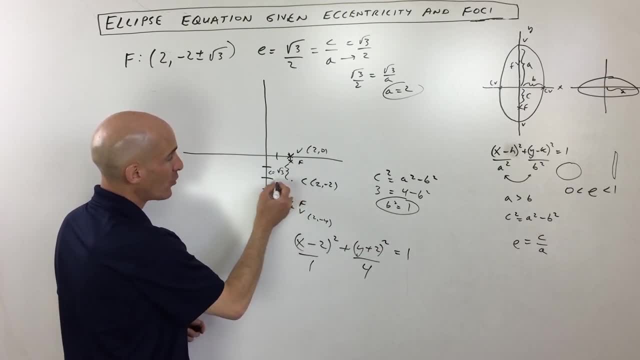 square root of 1, we still get 1. so the direction in the horizontal direction, okay, to the co-vertices, that distance is going to be 1. so you can see, here we've got a pretty good sketch of our ellipse and this is the equation, this is what we were trying to solve for originally and that wraps. 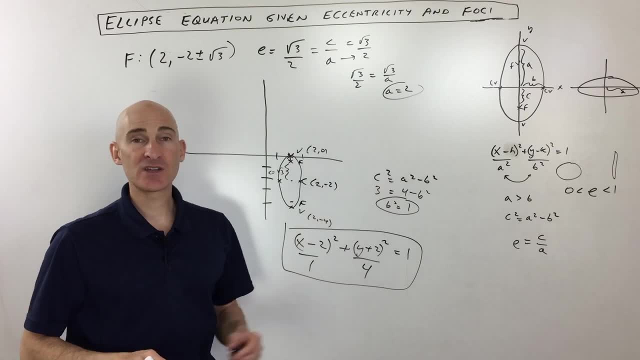 it up. so you Again. if you want to learn more about ellipses, I'll have links to other videos. I did talking about some of the more basic and general ones, but subscribe to the channel. check out more math tutoring videos on my YouTube channel. 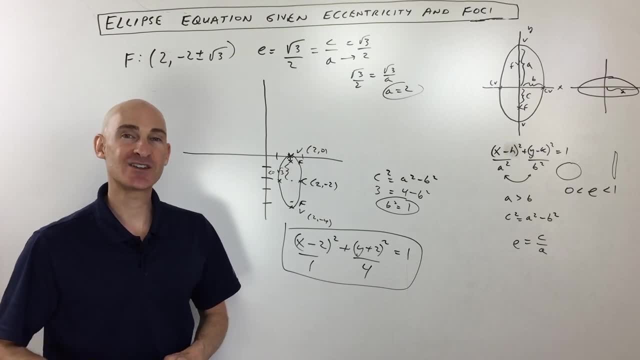 Mario's Math Tutoring and I look forward to helping you in the future videos. I'll talk to you soon.